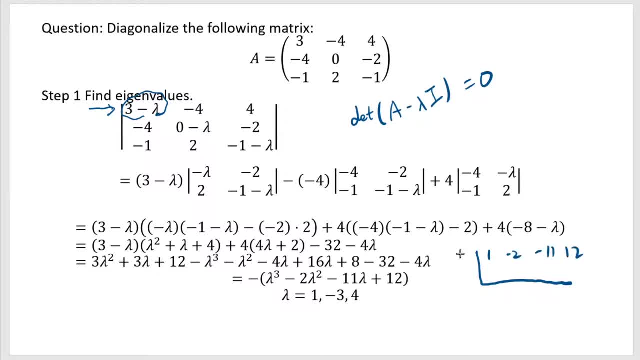 put 1 negative, 2 negative, 11, 12, then you put 1. 1 comes down 1 times. 1 is 1 negative, 1 negative, 1 negative, 12 negative. 12 goes to 0. so this is called synthetic division. it's really handy. so if you don't know that, please review it. 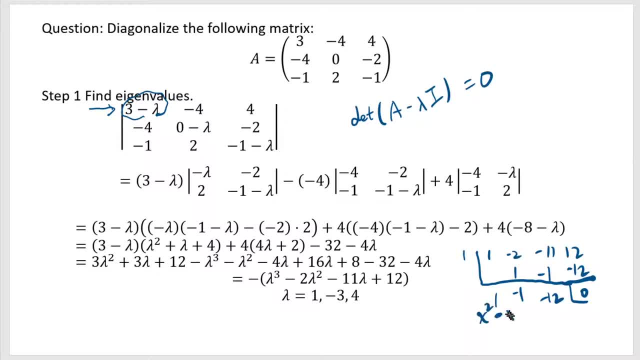 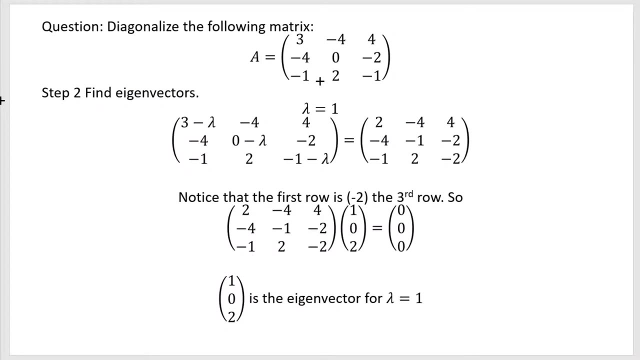 and then this one represents x squared minus X minus 12, so that also factors as a X minus 4, X plus 3. so that's how you get these answers. okay, now, once you get all the eigenvalues- remember we got the lambdas 1 and negative, 3 and 4- you have to find the eigenvectors and eigen. 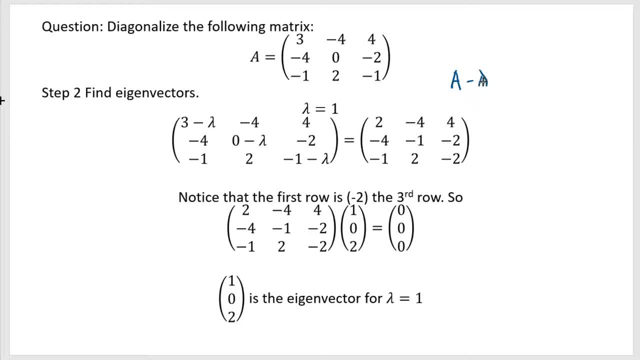 vectors are like vectors where, if you replace lambda by the values that we just obtained, we want to find vectors where this times this gives you 0, so we plug in 1 to this a minus lambda, I and you get this matrix. and to solve this time, 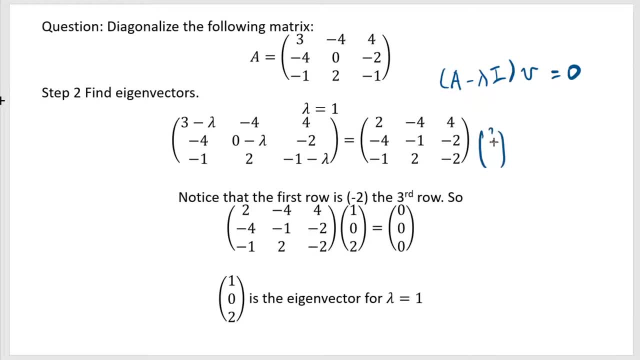 some vector equals to 0, something in here. sometimes you need to to look further, but sometimes the answer is right. right there. see, if you multiply this third 1 times 2, it's exactly same as the negative of this one. right? so you can see that if you multiply 1 0, 2, this gives you 0 0 0. so we find that 1 0 2 is. 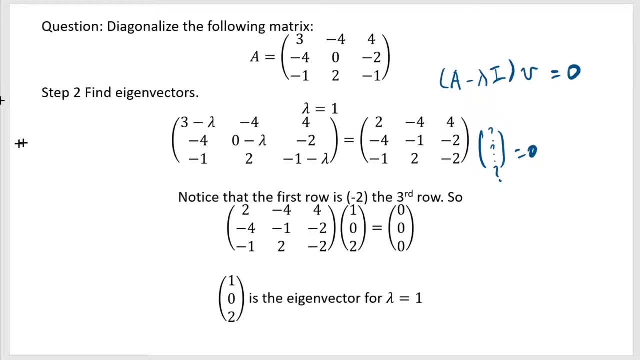 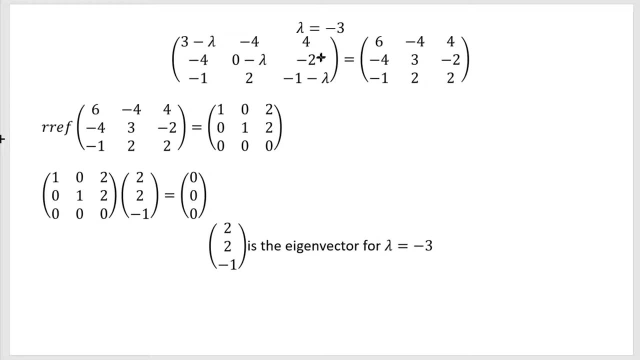 an eigenvector for lambda equal to 1. okay, next we need the following: lambda equals to negative 3. you plug in negative 3 and this time the problem is I don't see any such simple relationship, so this is a little bit more involved. in that case, what you can do is you can take the row. 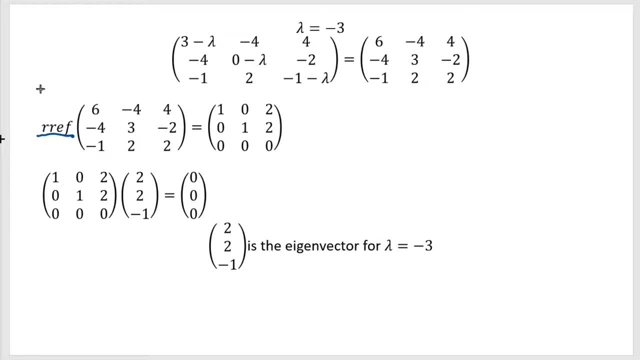 reduced echelon form. okay, so this is row reduced echelon form And you do this. you turn into reduced echelon form by making use of the Gaussian elimination, And that's also very basic stuff in matrices. So if you don't know that, you should review that as well. 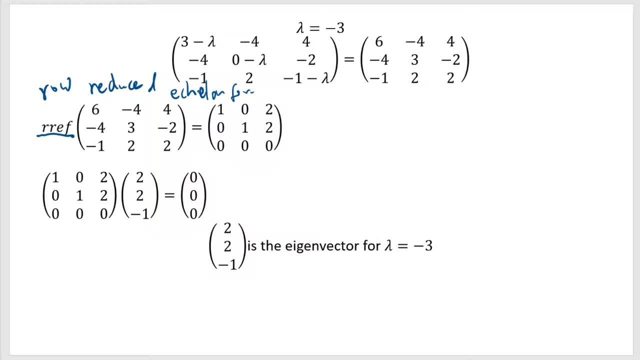 You could do this by hand, It's not that bad. But since the goal is just to demonstrate how this entire thing is done, I'm going to use this website, where it's something in emathhelpnet. I just googled RREF calculator and it got me to this. 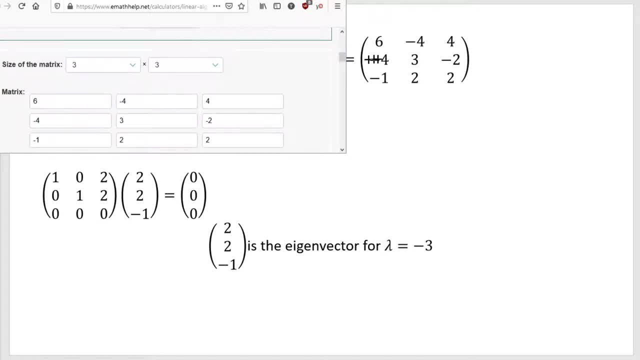 And you just choose the size of the matrix, And I just plugged in the value 6, negative 4,, 4, and all that, And I click calculate. And not only does the calculation, it shows all the intermediate steps. So all the intermediate steps are shown. 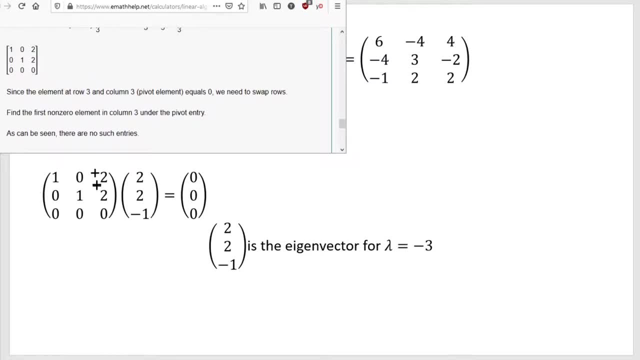 And this is the final row-reduced echelon form. The important thing is, if you have something times ABC equals to 0, where this is supposed to be this, even if you do the row reduction, row-reduced echelon form. 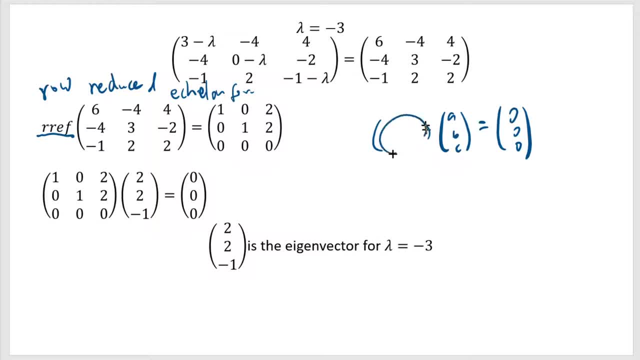 the equation still is true, So you can replace this by its RREF. That's the trick. So we We have this times some matrix. ABC equals to 0. And that means 1 times A plus 2 times 0 times B plus 2 times C equals to 0.. 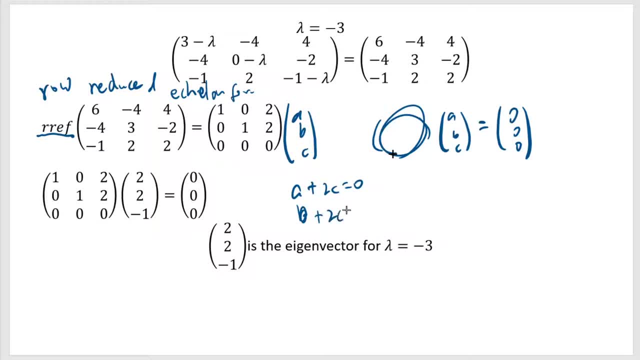 And 1 times B plus 2C equals to 0. So if you set C as negative 1, then A and B will be 2.. So that's one solution After all. we're just trying to find one solution, not all solutions. 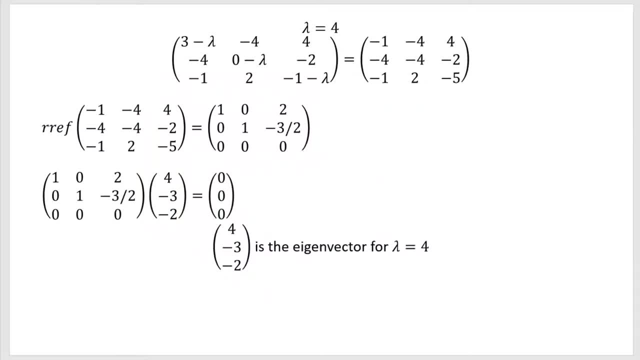 So we got the next eigenvector. Now let's move on. Do the same thing for lambda equals to 4.. Calculate the RREF And then think about what that means, And we find that this is the eigenvector for lambda equals to 4.. 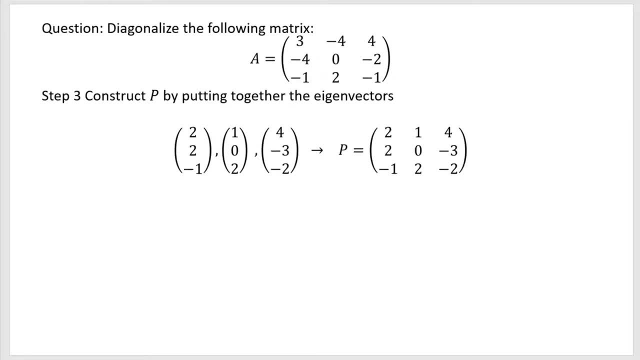 Once you get these, then what you can do is you write all the eigenvectors you found and place them side by side, And that's going to be your P, And using this, we are going to diagonalize this matrix. So let me show you how that's done. 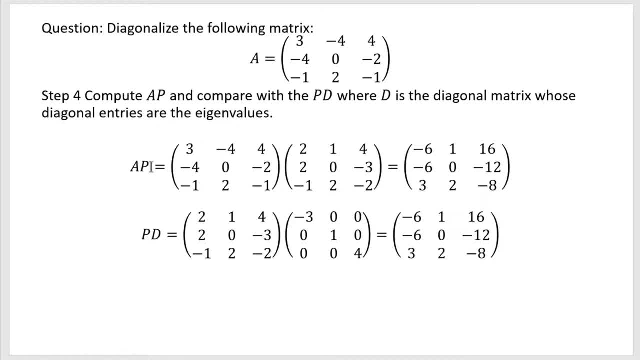 What you want to calculate is AP and PD, where D is the matrix. It's a diagonal matrix with eigenvalues on the diagonal. Okay, All right, So you can actually do this calculation And, if you trust me, what happens is because this part right here is an eigenvector. 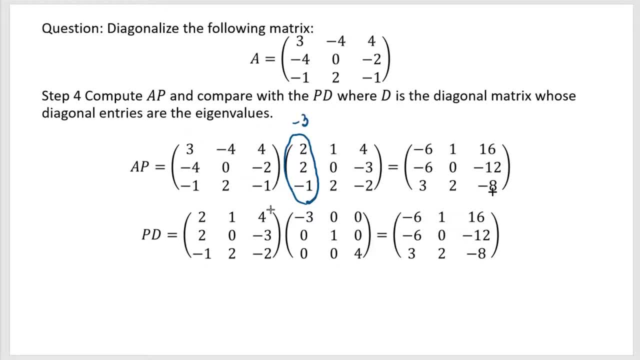 with eigenvalues, It's going to give you negative 3, and this one had 1, and that was 4.. What you end up is, if you multiply this matrix to this, it will just give you this, which is: this is really negative 3 times 2 to negative 1.. 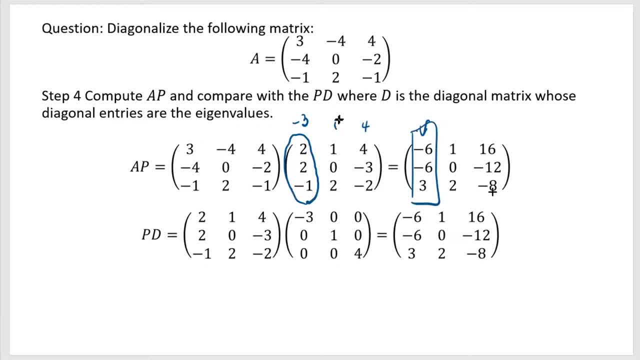 Okay, So this is negative. 3 times this, So, and then 1 times 1,, 0,, 2 is this and 4 times this will give you that. Okay, So you can check the actual calculation. Okay, So you can check the actual calculation. 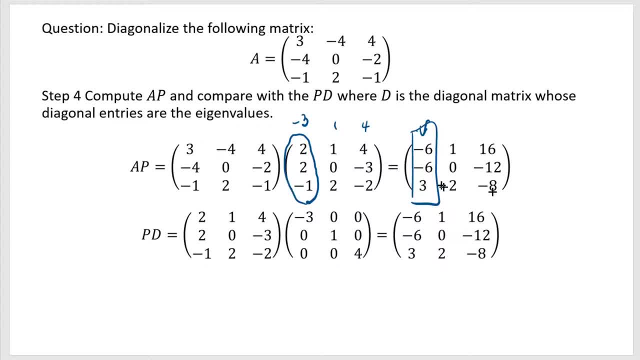 Okay, So you can check the actual calculation. You don't trust me, but if you actually do, you will find that the matrix you get will be, column-wise, the result of what you would get if you think about the eigenvector equation. 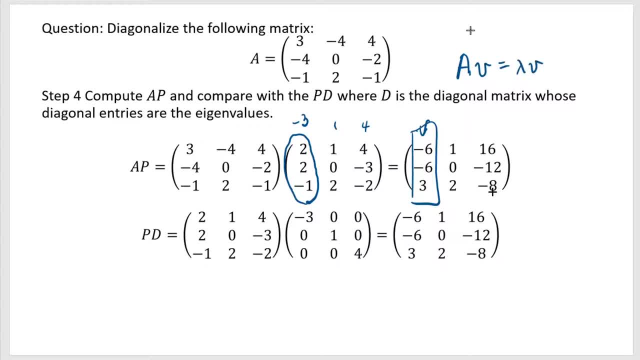 Eigenvector. I mean, this is equal to saying A minus lambda. I times V equals to 0.. Right, So using this relationship, you can verify all these. Okay Now, furthermore, if you multiply these two matrices, what happens is that, if you have a diagonal matrix, 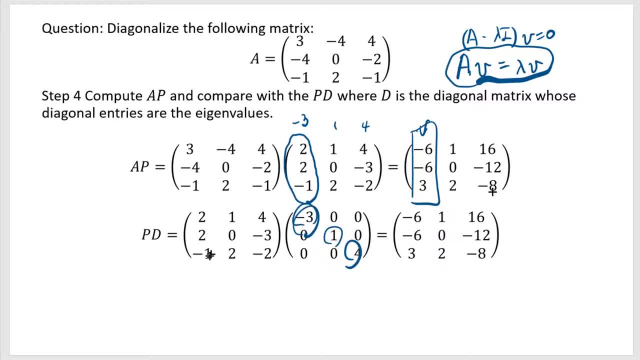 with some numbers like that. this makes the entire first column to be multiplied by negative 3.. So you get this. One makes the entire second column to be multiplied by 1.. Four makes the entire third column to be multiplied by 4.. 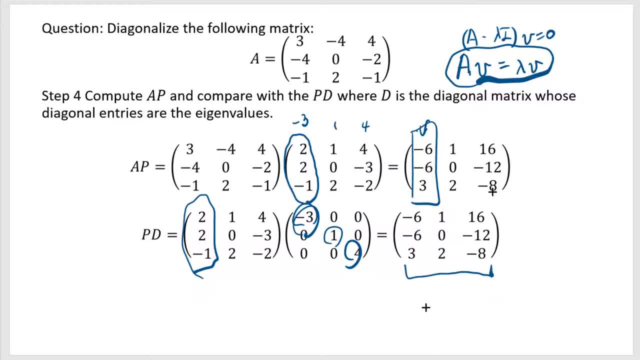 So again, you get the same effect. Okay, And now? this is a very interesting conclusion, because what we just verified is that AP is equal to PD, So AP equals to PD And therefore, if you multiply P, inverse both sides, these two will cancel. 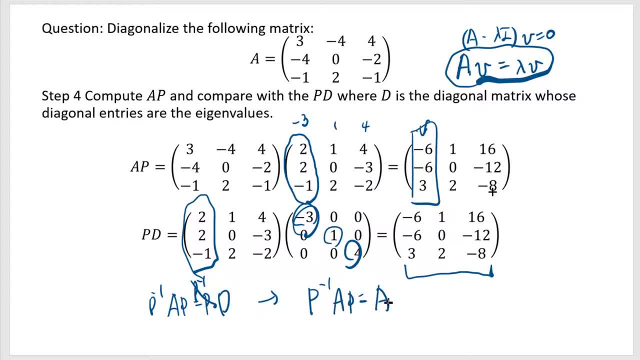 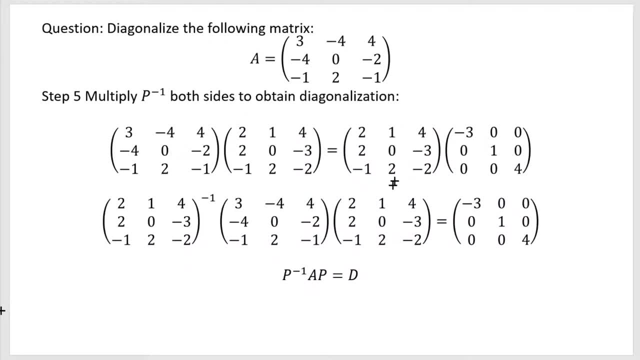 and you end up with P inverse. AP equals a diagonal matrix. Okay, So in our specific case, we have proved that there's identity between these two and this is our matrix, P, And if you take the inverse of this, you get the P inverse A times P equal.